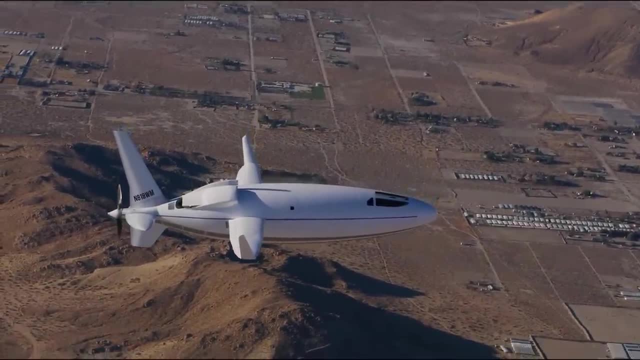 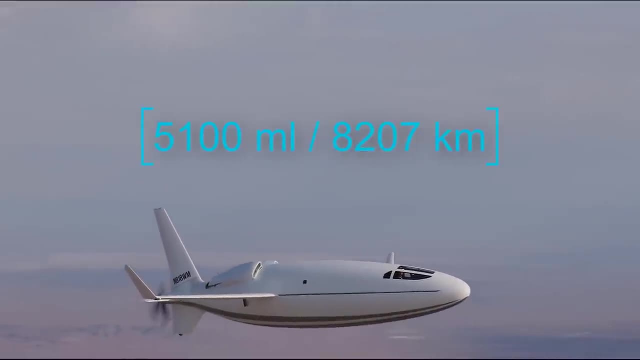 This enables a massive leap in efficiency, speed and range compared to traditional plane geometries. Celera can cover a distance of about 5,100 miles, which is more than enough to travel, for example, from Alaska to Mexico using 80% less fuel than a comparable. 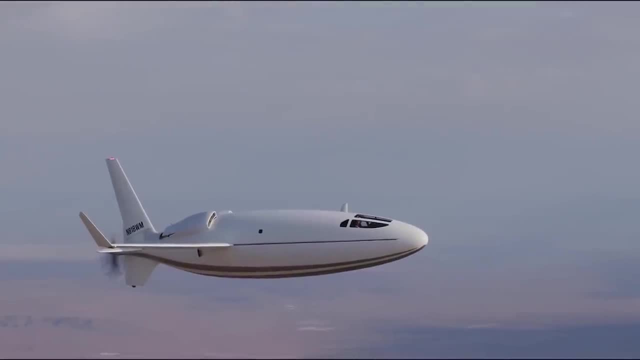 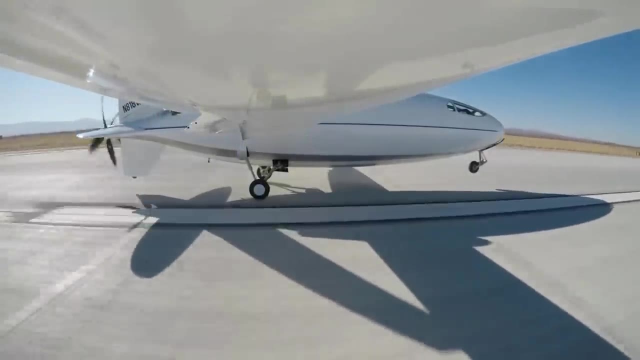 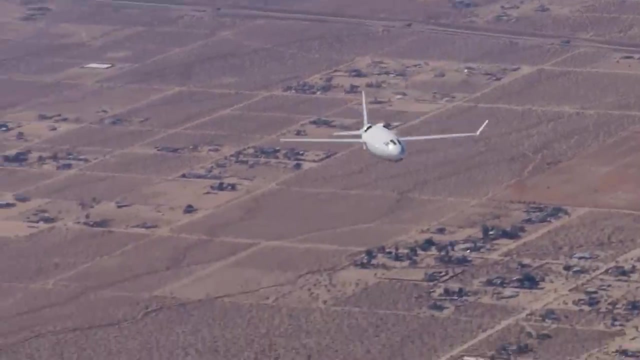 airplane. Besides, Otto doesn't use the wings to store fuel. The long and skinny wings are to provide maximum lift and minimum drag, due to which it has reached an impressive glide ratio of 22 to 1, allowing pilots to switch off the engine altogether and glide. 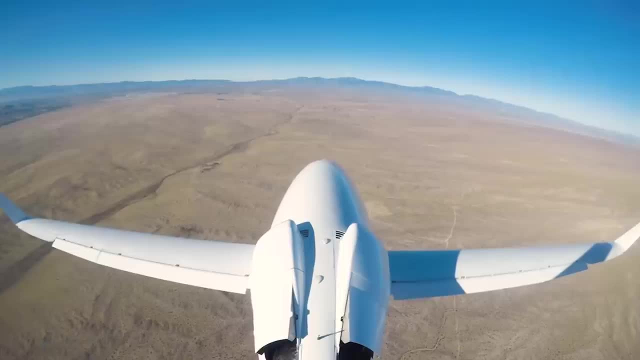 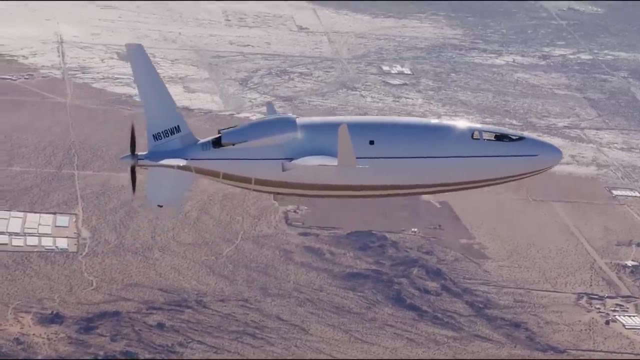 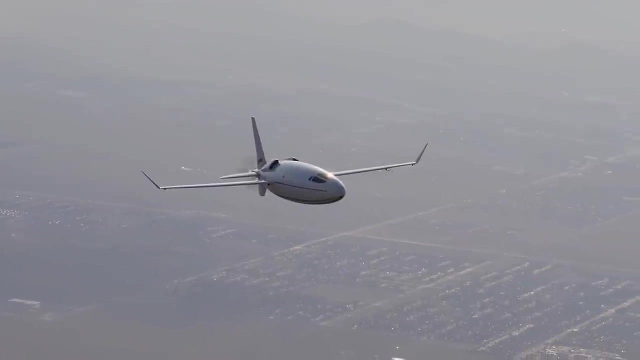 unpowered for up to 125 miles, which the company says is roughly three times better than the typical aircraft. The airplane's excellent aerodynamic design enables reaching high-speed and altitude without using expensive jet engines To match its most efficient aerodynamic body. 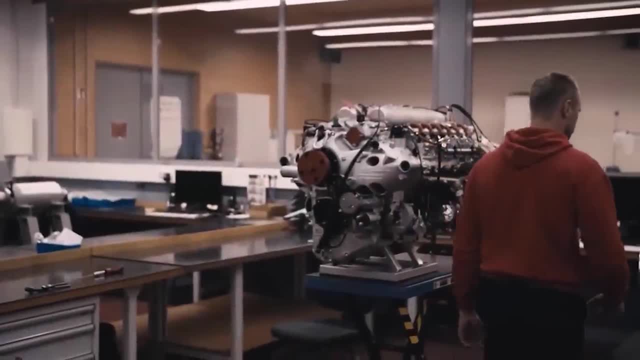 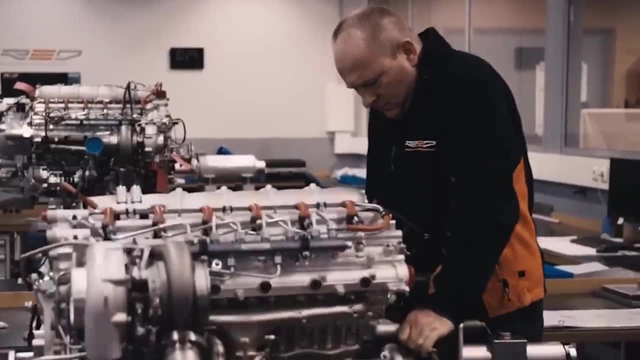 the Celera 500L is equipped with a single turbocharged V12 diesel engine at the back, designed by German manufacturer RED. The position of the piston engine helps prevent the laminar flow from distorting and provides better acceleration, Because laminar flow makes the 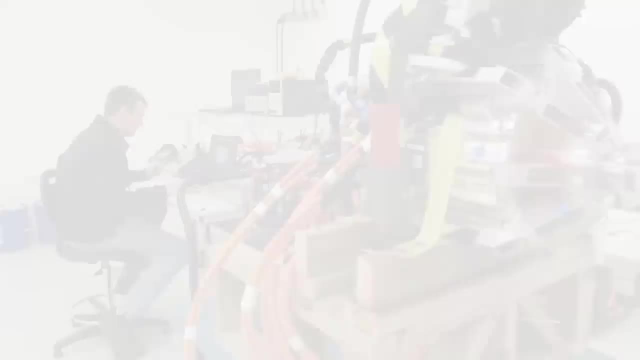 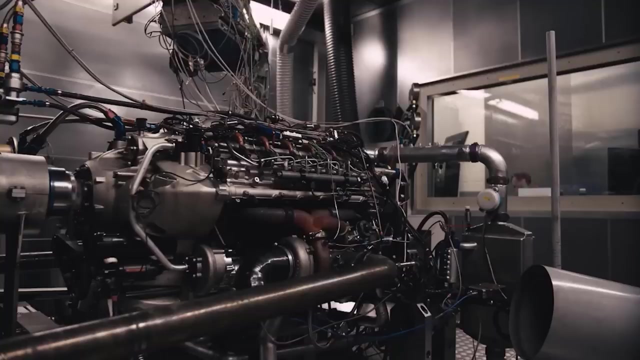 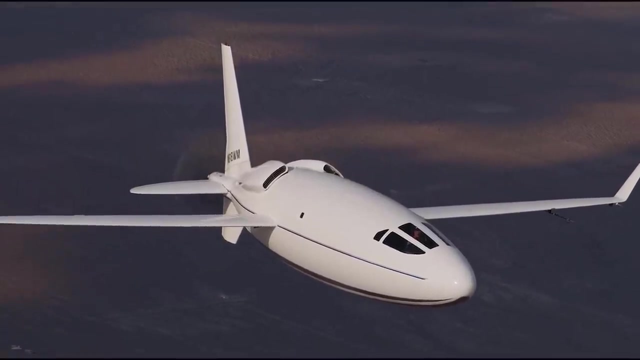 plane require less energy. the engine bay could be filled with an electric motor, which we'll get to shortly in the video. The engine is expected to eventually be able to push the airplane up to 460 miles per hour at 50,000 feet, which is an excellent result for an affordable aircraft. 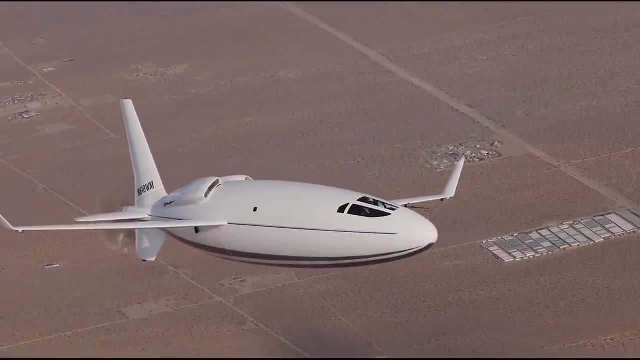 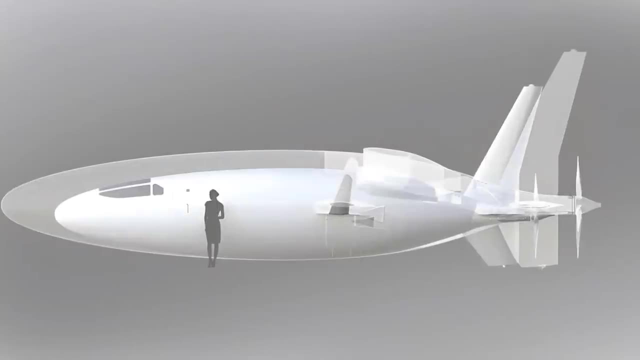 Since Celera's design benefits will not scale upwards to full-size airliners. the initial version of the plane is designed to carry six passengers in a business cabin, scalable to 19 passengers later on, And with a running cost of $328,. it will be five times more. cost-effective than the original Celera 500L. The engine is expected to eventually be able to push the plane up to 460 miles per hour at 50,000 feet, which will be five times more cost-effective than BizJets with comparable performance and comfort. 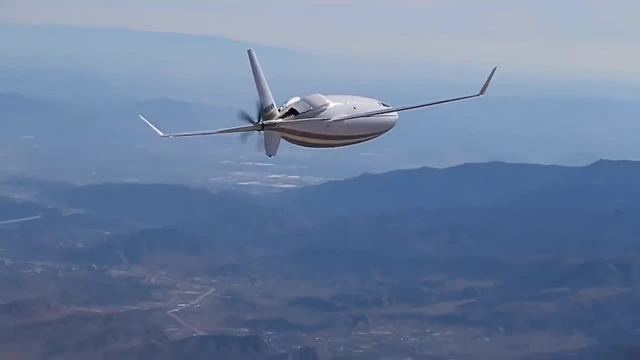 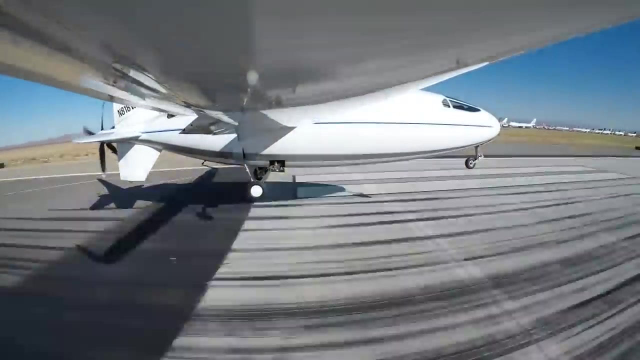 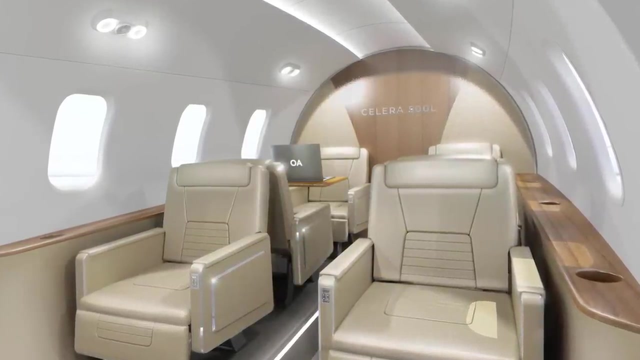 In the end, the goal of this amazing project is to create an aircraft that would allow for direct flights between any city pair at speeds and cost comparable to commercial airfares, but with the added convenience of private aviation. It offers a spacious stand-up cabin with first-class seats and a lavatory. 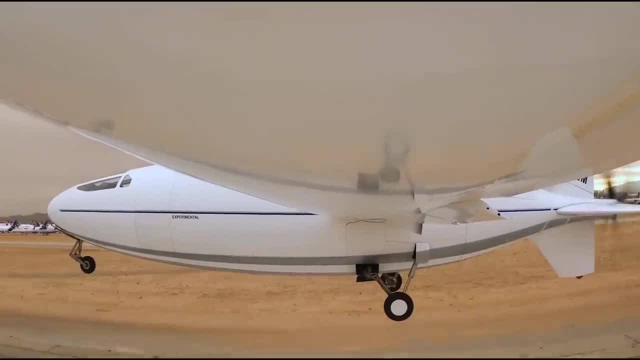 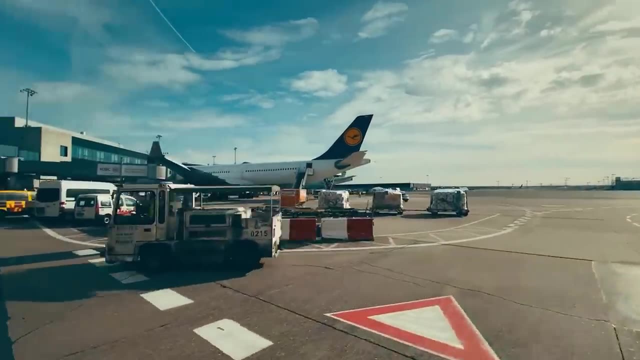 Celera needs a short take-off length, which means it will have direct access to over 5,000 regional airports. Celera 500L is the first-class aircraft in the world to be able to take off from the airport, Unlike commercial airlines that serve only about 500 airports in the US.